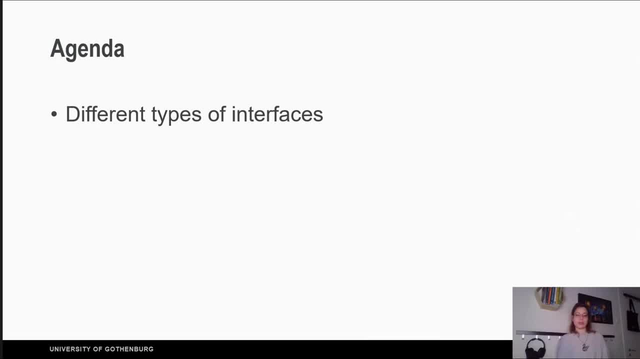 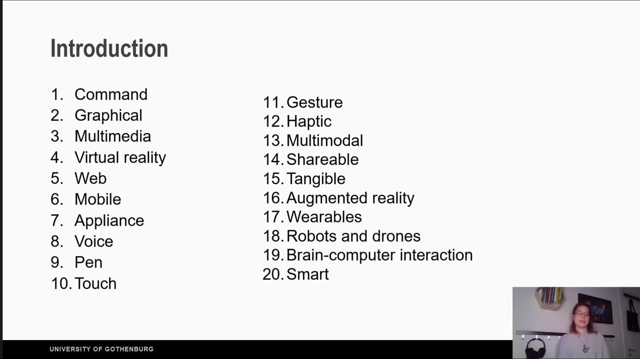 Gothenburg in the Applied IT department on Human-Computer Interaction. we are not expect you to memorize every example of this chapter, but we expect you to be able to recognize the different types of interfaces. In this chapter we will see 20 interfaces: Command, Graphical Multimedia. 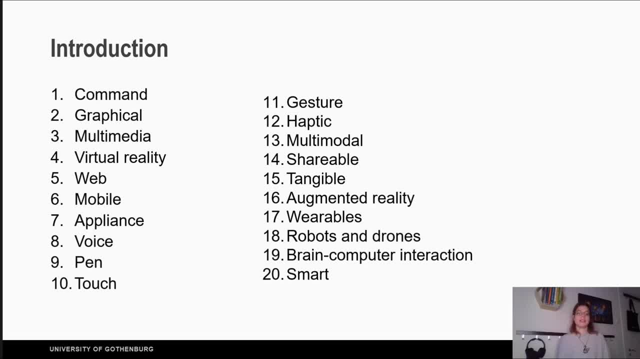 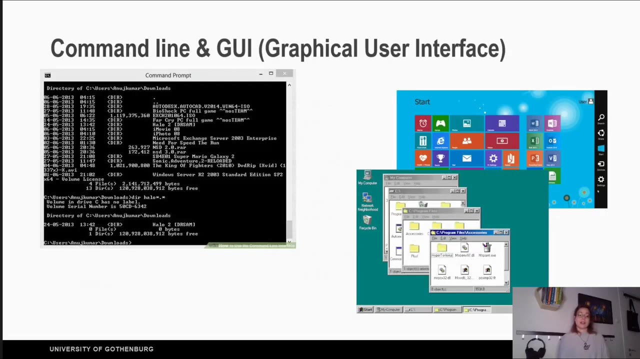 Virtual Reality Web, Mobile Alliance, Voice, Pen, Touch, Gesture, Haptic, Multimodal, Shareable, Tangible Augmented Reality, Wearables, Robots and Drones, Brain-Computer Interaction and Smart. Let's start with the command line and graphical user interfaces: GUI. 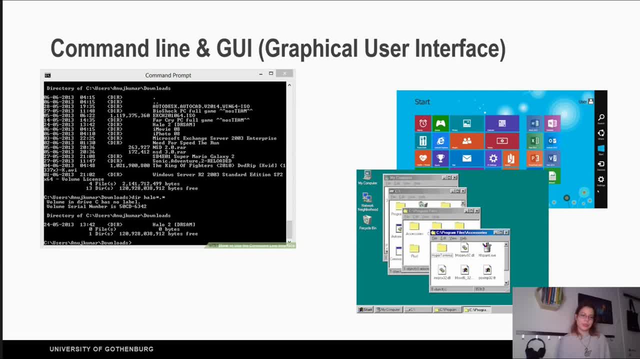 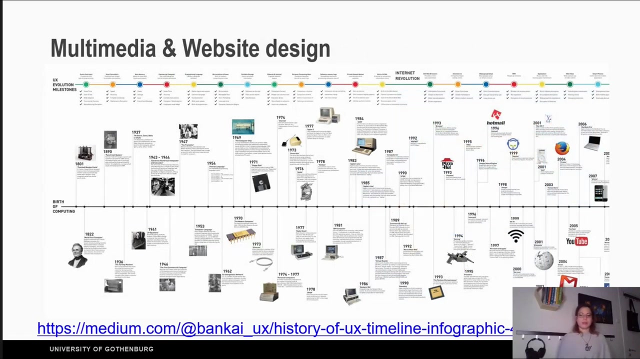 The first interaction with the one of the first interactions with the computers were by typing commands in a command line in order to access different files. Later we had the graphical interface, where windows folders and other files took a visual form: Multimedia and web design. Multimedia involve more than one way of presenting information. 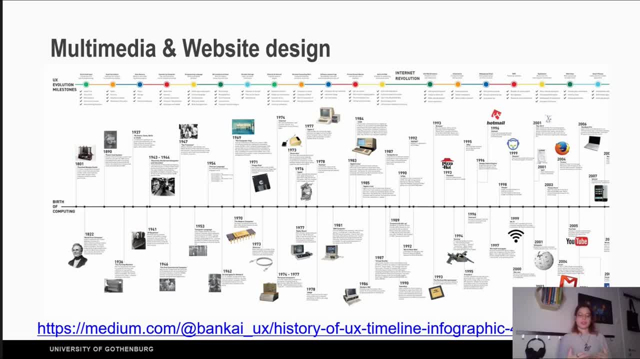 it's really important because it can give different ways of accessing the same information: visual, auditory or even written. the picture underneath. i don't expect you to be able to read it, but you can follow the link in the description of this video to see the development of. 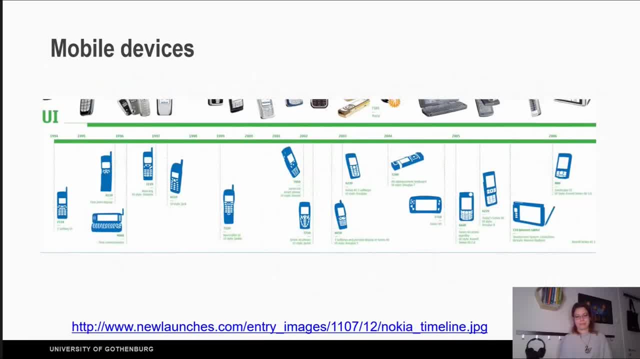 web design. here we can see the development of ui in mobile devices. please follow the link in order to see the image in more detail. and we should not point out that the mobile devices nowadays are pervasive. everywhere we go, we may have a smartphone with us, some kind of wearable and some kind of fitness. 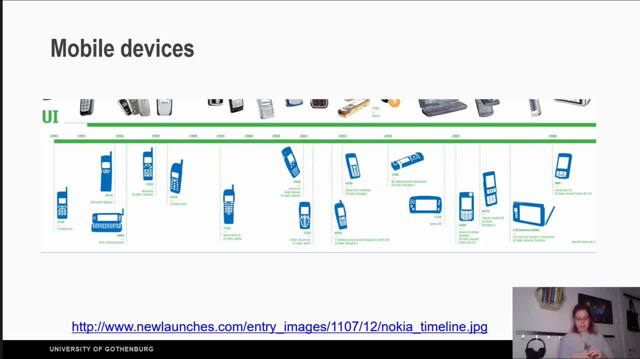 trackers, like here. i have the aura ring, which is a wearable ring that can measure your temperature, your breathing, and can give you data about your sleep. so there are all those device. devices are mobiles, even the laptops, which are bigger but still mobile. appliances is every appliance that? 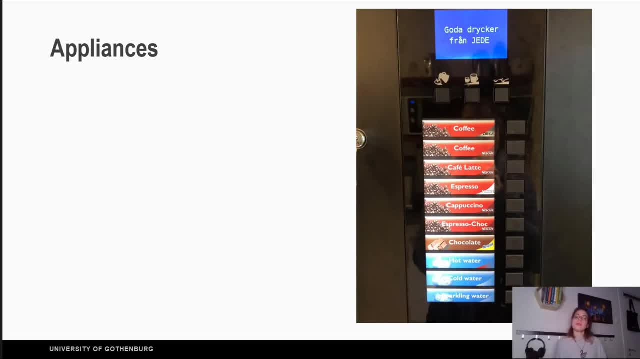 has digital interface here. I would like to show you a little bit more about what we have here. inside the cover story of young alert, you can follow the link in order to read the full story. it writes: you are likely familiar with the following situation: standing in front of a 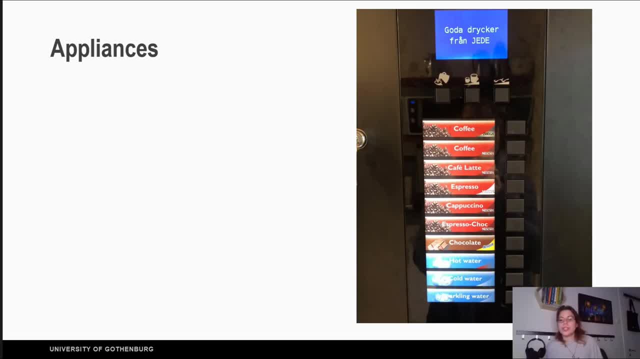 coffee machine, you're uncertain whether you should just press the coffee button momentarily or if you are supposed to keep pressing it until your cup is filled. the second button option is like a buzzer: coffee keeps pouring only as long as you press. the first option, however, is at least as likely in a modern machine. 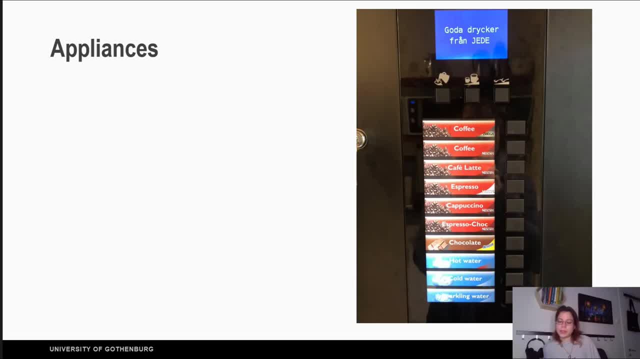 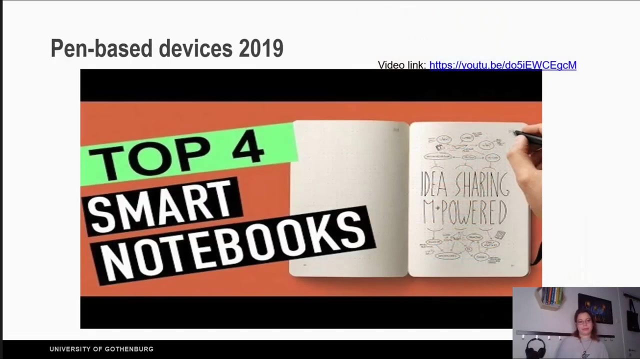 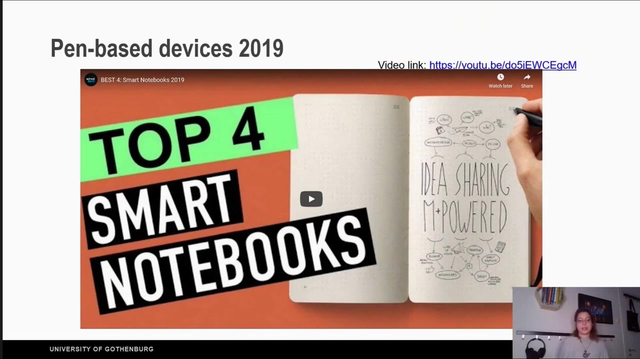 initiate a process that will be automatically completed, rather than continuously controlled the process yourself. without disputing the benefits of automation, one may wonder how, such modern days, uncertainties arose. might the last development of the bottoms- bottoms themselves- have something to do with it? here is a video that can show you a pen based devices of. 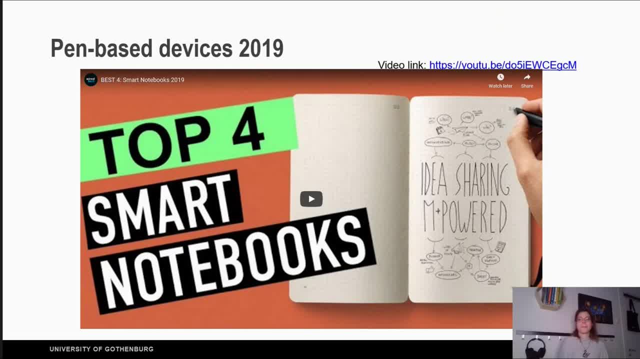 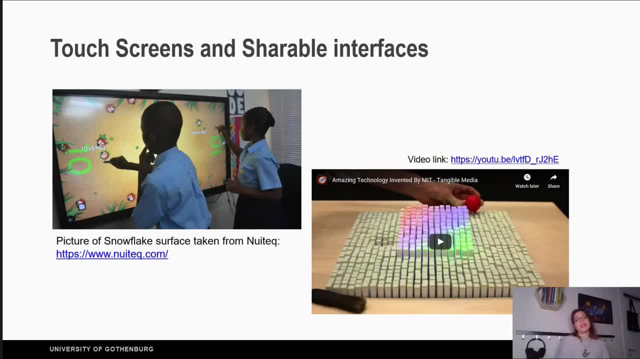 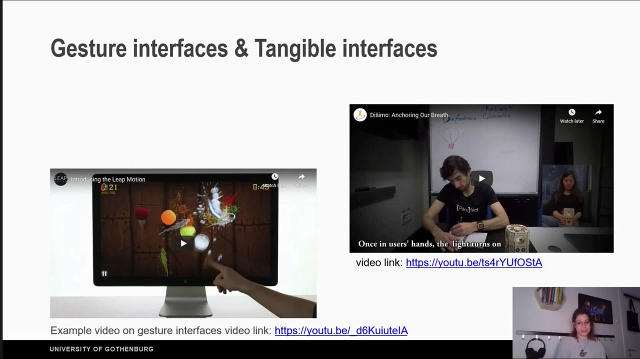 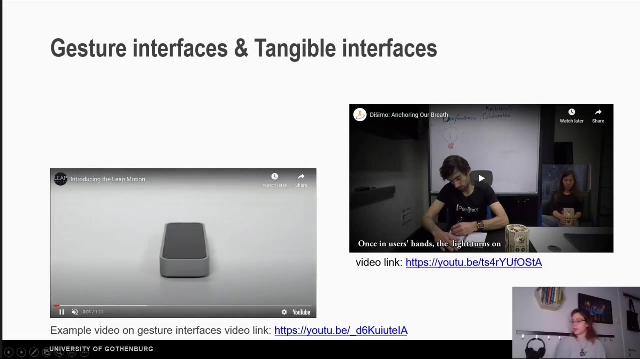 the a コ cross, cross, cross episode is the first discussed. this is done in the class a at tangible cerebral interface, gestures and tangible interfaces. so in this video we can see leap, where it's a small device that you put it in front of your screen and then you can start controlling your computer by using gestures. however, 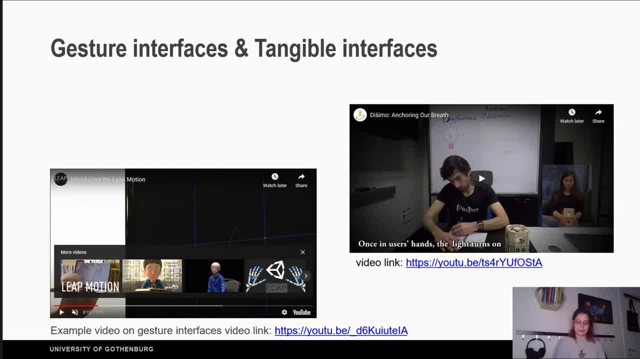 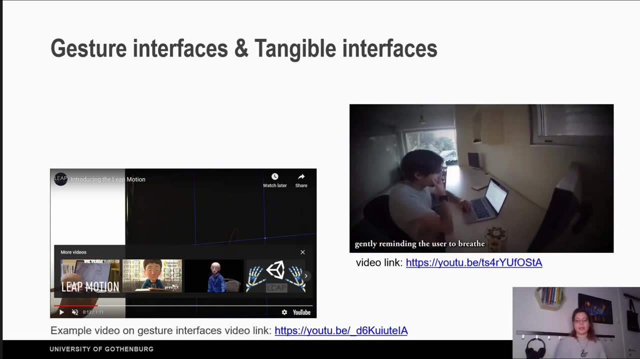 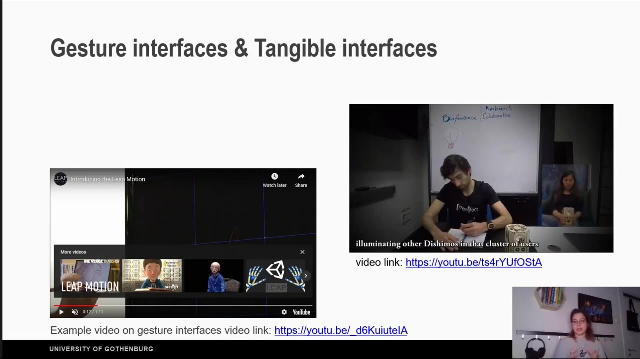 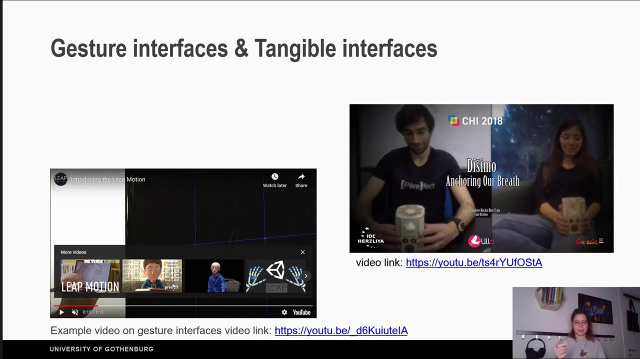 gestures are not socially acceptable in all the cultures. tangible interfaces. in this video you can see thisgmo. this move is this wooden machine that it makes a sound. when a person- that's the machine, the other person that's also the machine, and when their breathing are aligned, then these things inside the wooden box start moving. 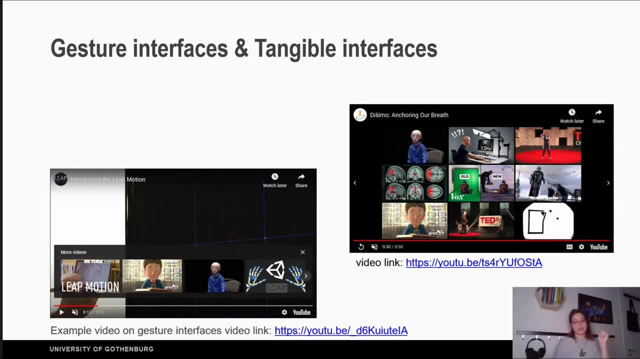 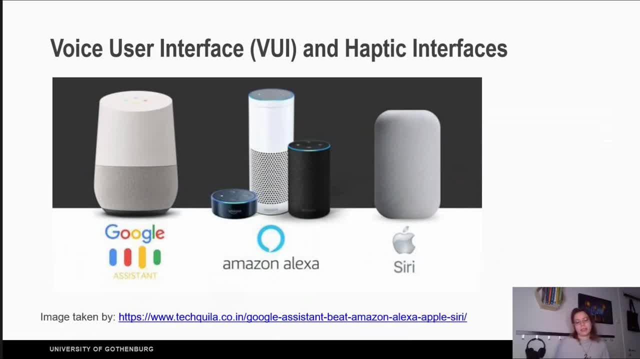 You can feel free to watch the video alone by clicking the link in the description. Voice interfaces and haptic interfaces. Voice interfaces: we talked a little bit about them in previous chapters, and it's when we talk to a computer like: hey, Google, what is the weather? 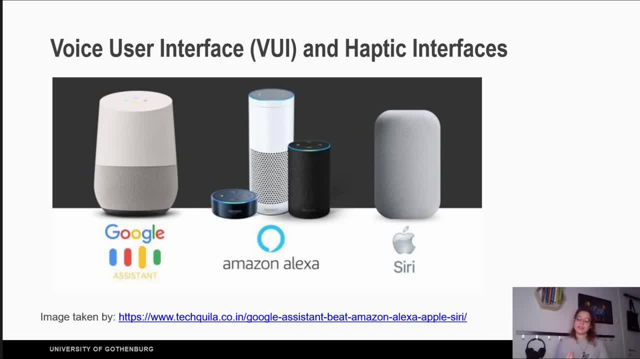 today, Haptic interfaces is when the device that we are attaching give us a feedback, a tactile feedback. For example, if you go to the Google assistant and try to adjust the volume, from the top of the assistant, you will feel a small vibration that shows that. 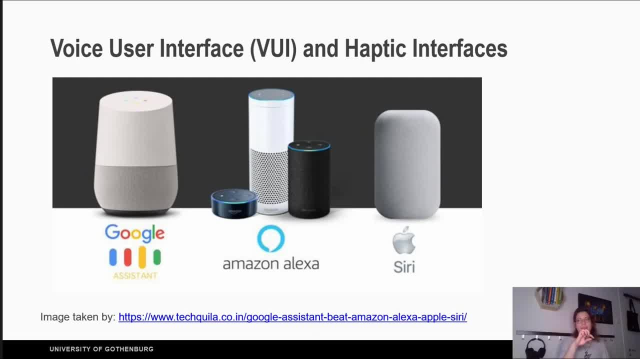 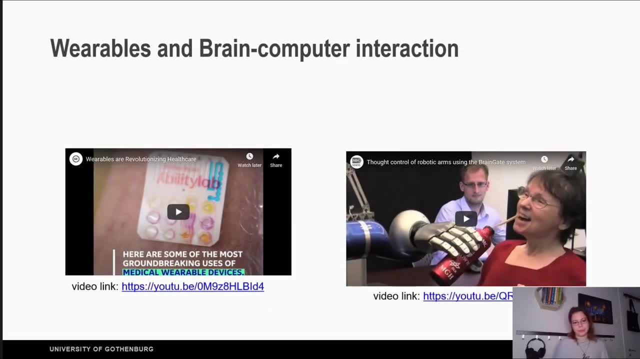 you go through the different levels of value: Wearables and brain computer interaction. Wearables is technology that we can wear. It's a mobile technology and, as I showed before, it can take the form of a ring. it can take a form of the pads. Feel free to watch the video about a medical